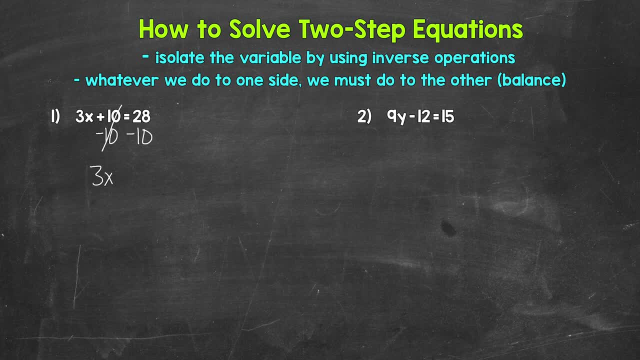 So we are left with 3x equals. And then on the right side of the equation we have 28 minus 10, which gives us 18. So now we have 3x equals 18. We are multiplying x by 3.. 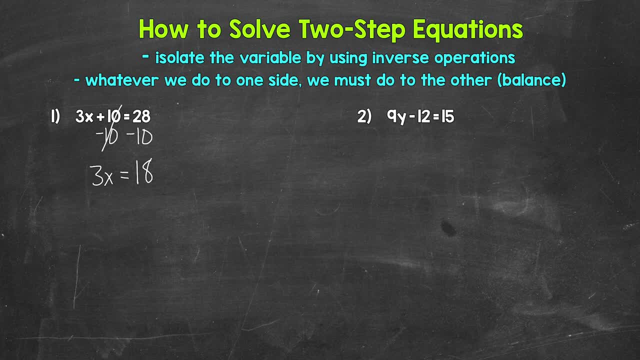 So we need to undo, We need to do that, We need the inverse operation here in order to isolate x. The inverse operation of multiplication is division. So let's divide the left side of the equation by 3.. Whatever we do to one side, we must do to the other. 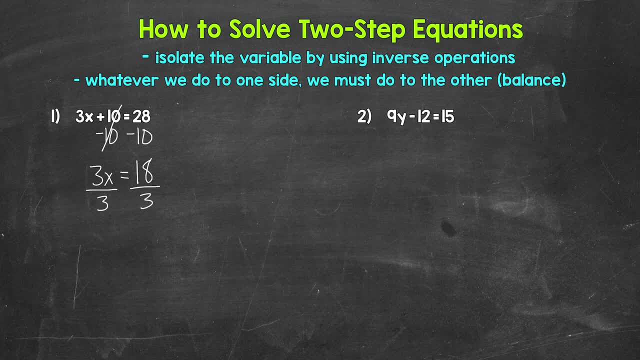 So divide the right side by 3 as well. On the left side of the equation we are multiplying by 3 and dividing by 3.. So these 3s Cancel each other out. Now our variable x is isolated, So we have x equals. 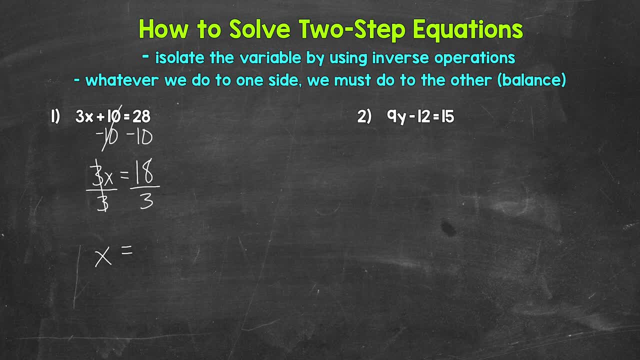 And then on the right side of the equation, 18 divided by 3 is 6.. So x equals 6.. And that's our solution. Now one last thing we can do. We can always check to see if we are correct. 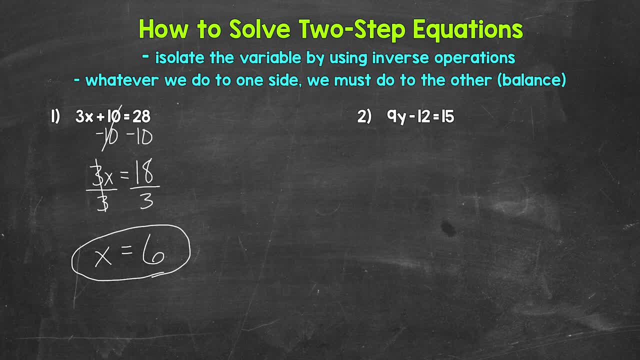 And we do that by plugging in what we got And seeing if it works. So, for example, let's plug in 6 for x and see if it works. So we can come to the side here. 3 times 6 plus 10 equals 28.. 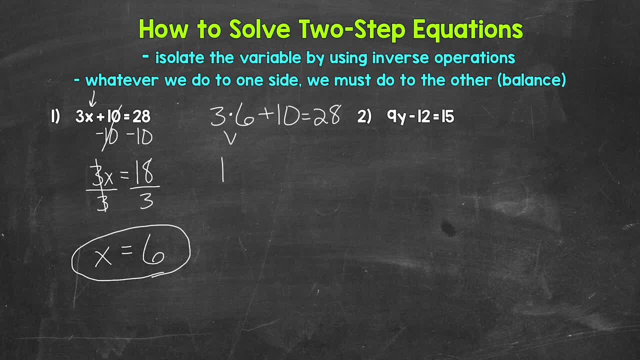 So we need to multiply first 3 times 6 is 18.. So we have 18 plus 10.. 18 plus 10 is 28.. So we are correct: x Equals 6.. Let's move on to number 2.. 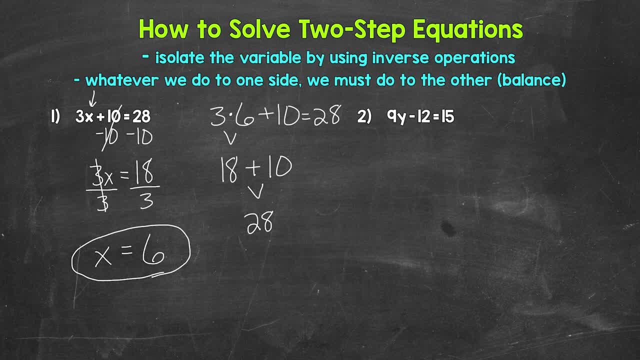 Where we have 9y minus 12 equals 15.. So 9 times what minus 12 equals 15.. We need to isolate that variable of y. We need to undo the operations. on that side of the equation We have multiplication and subtraction. 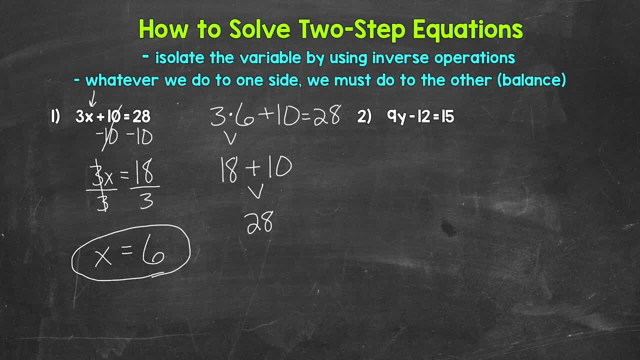 So we need to go in the reverse order of operations in order to undo everything Here. we need to undo the subtraction first. So what's the inverse operation of subtraction? Well, addition. So let's add 12 to the left side of the equation. 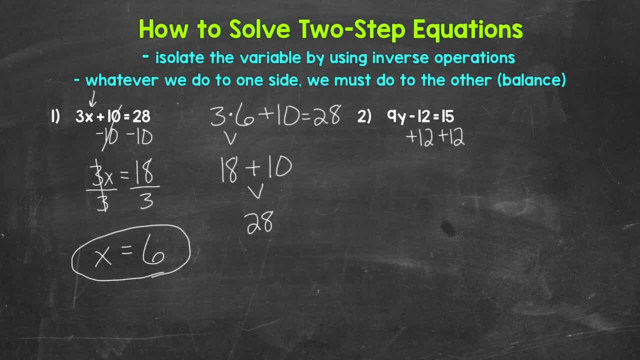 Whatever we do to one side, we must do to the other. So add 12 to the right side as well. On the left side, we are subtracting 12 and adding 12.. So these 12s cancel each other out. 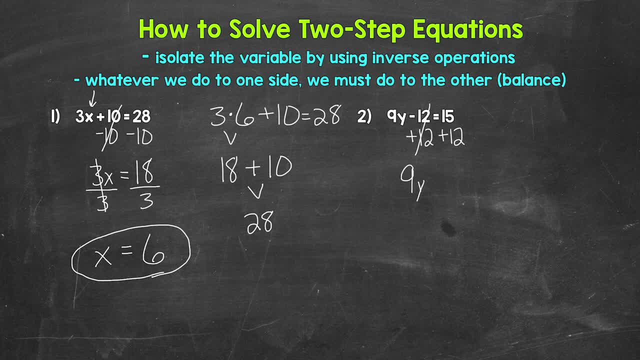 So we have 9y equals. And then on the right side of the equation, 15 plus 12 gives us 27. So now we have 9y equals 27. So we're multiplying y by 9. And we need to undo that multiplication by using the inverse operation. 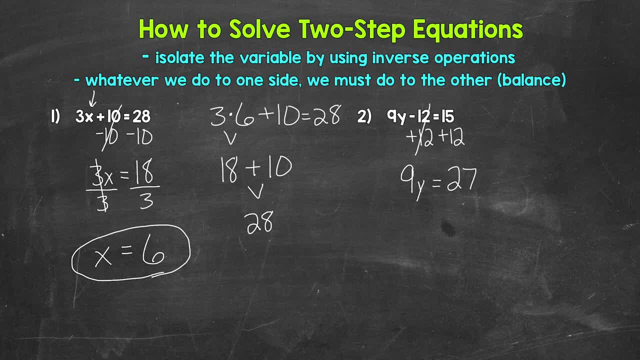 What's the inverse operation of multiplication? Well, division. So let's divide the left side by 9.. Whatever we do to one side, we must do to the other. So divide the right side by 9 as well. On the left side, we are multiplying by 9 and dividing by 9.. 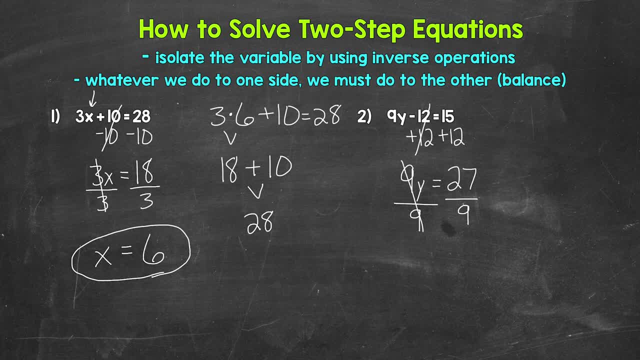 So these 9s cancel each other out And our variable y is now isolated. So we have y equals. And then on the right side of the equation we have 27 divided by 9. Which gives us 3.. 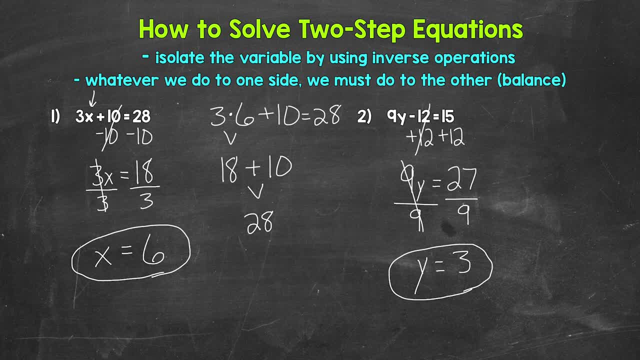 So y equals 3.. And that's our solution. Now let's plug it in and see if we are correct. So plug in 3 for y. So 9 times 3 minus 12 equals 15.. So we start with multiplication. 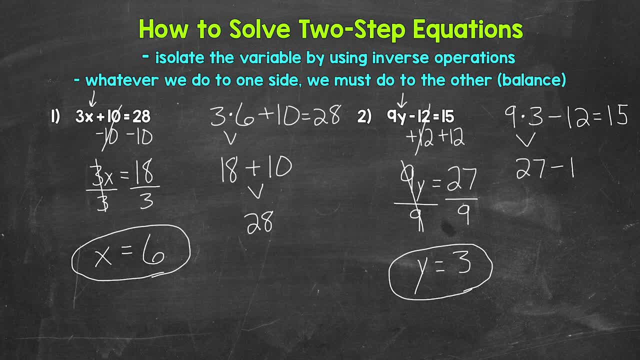 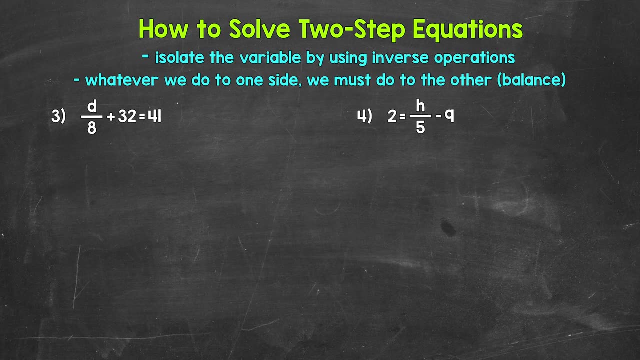 9 times 3 is 27.. 27 minus 12 is 15.. So we are correct: y equals 3.. Let's move on to numbers 3 and 4.. So here are numbers 3 and 4.. Let's jump into number 3, where we have d divided by 8 plus 32 equals 41.. 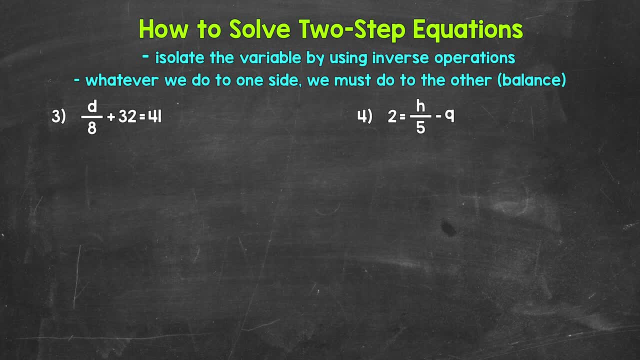 So we need to isolate that variable of d using inverse operations And we need to go in the reverse direction. So we need to go in the reverse order of operations. We need to undo the addition first. So what's the inverse operation of addition? 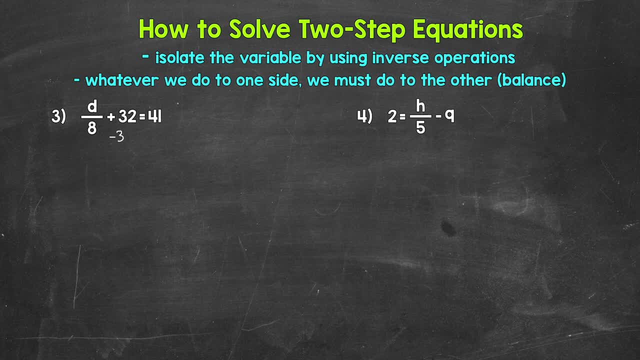 Well, subtraction. So let's subtract 32 from the left side of the equation. Whatever we do to one side, we must do to the other. So subtract 32 from the right side as well. Now, on the left side of the equation, we are adding 32 and subtracting 32.. 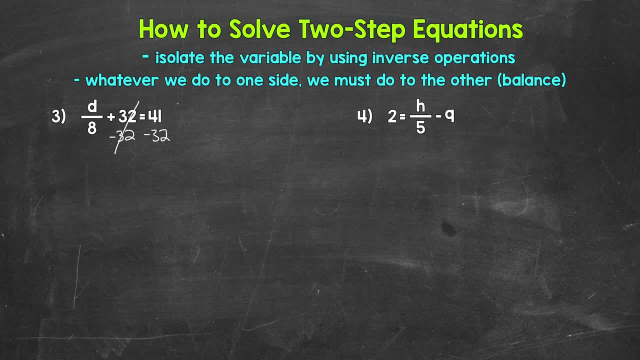 So we subtract 32.. So these 32s cancel each other out. So we have d divided by 8 equals. And then, on the right side of the equation, we have 41 minus 32.. That gives us 9.. So we have d divided by 8, equals 9.. 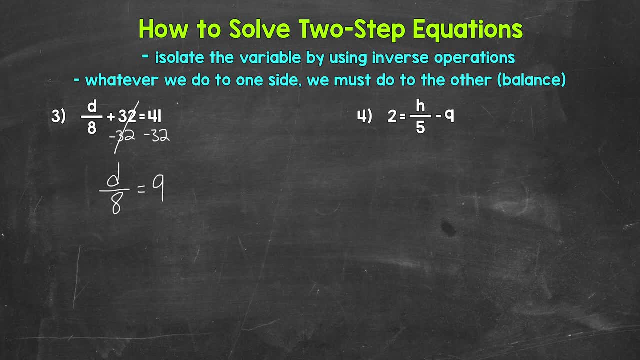 So let's continue to look to isolate that variable of d. So d is being divided by 8.. What's the inverse operation, The opposite of division? Well, multiplication. So let's multiply the left side by 8.. Whatever we do to one side, we must do to the other. 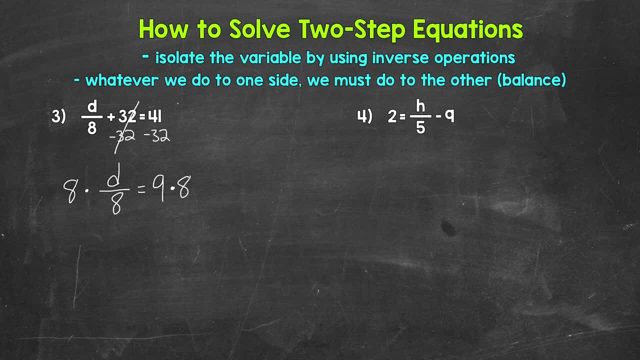 So multiply the right side by 8 as well. Now on the left side we are dividing by 8 and multiplying by 8. These 8s cancel each other out. So d is now isolated. d equals, and then on the right side, 9 times 8. 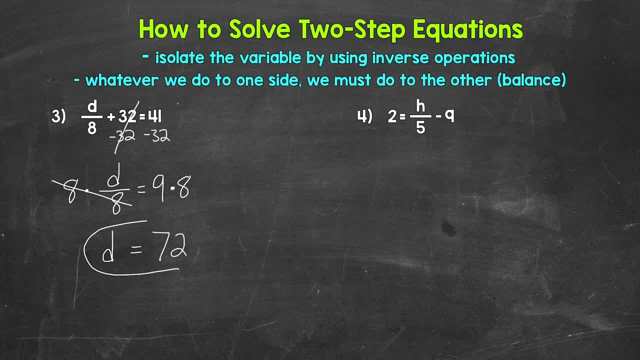 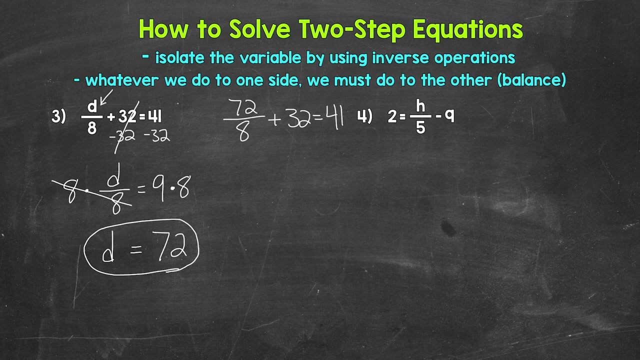 gives us 72.. So d equals 72.. That's our solution. And let's check that by plugging 72 in for d. So we have 72 divided by 8 plus 32 equals 41.. 72 divided by 8 is 9.. 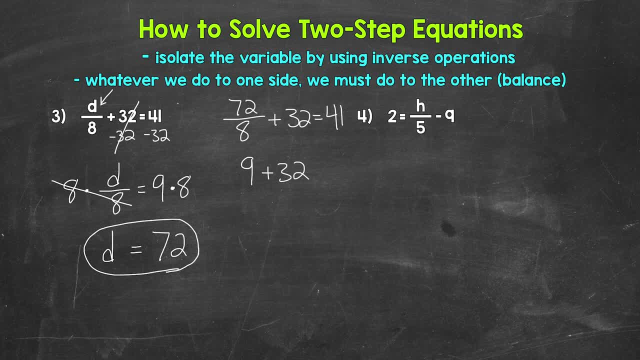 So we have 9 plus 32.. And that gives us 41. So we are correct: d equals 72.. Lastly, let's move on to number 4. Where we have 2 equals h divided by 5 minus 9.. 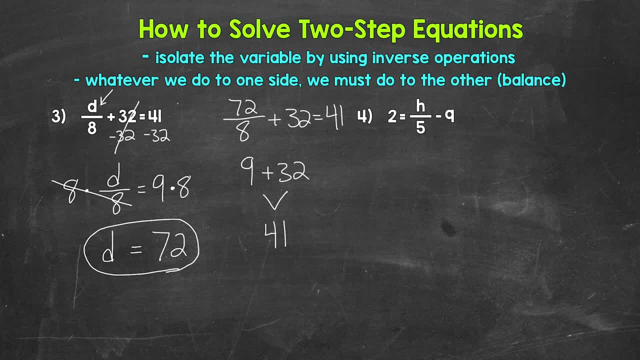 Now for number 4, the variable is on the right side of the equation, So a little bit of a different look here, But we use the same exact process, So this doesn't change anything. So we have 9 plus 32.. 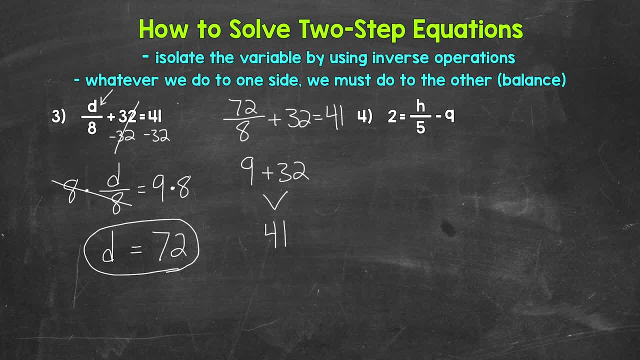 And that gives us 41. So we are correct: d equals 72.. So we are correct. So this doesn't change anything. So we need to isolate that variable of h. So h is being divided by 5.. And then we are subtracting 9.. 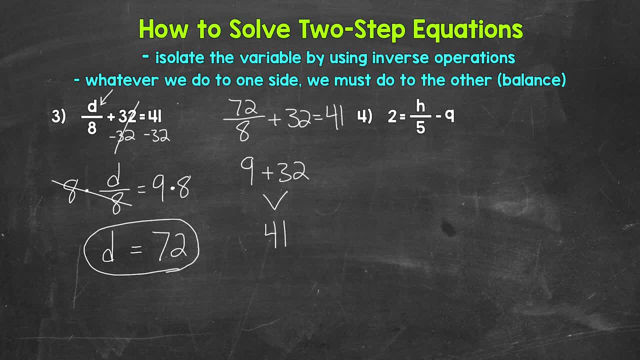 So let's undo that subtraction first. So let's undo that subtraction first. What's the inverse operation of subtraction? What's the inverse operation of subtraction? Well, addition. So let's add 9 to the right side of the equation. So let's add 9 to the right side of the equation. 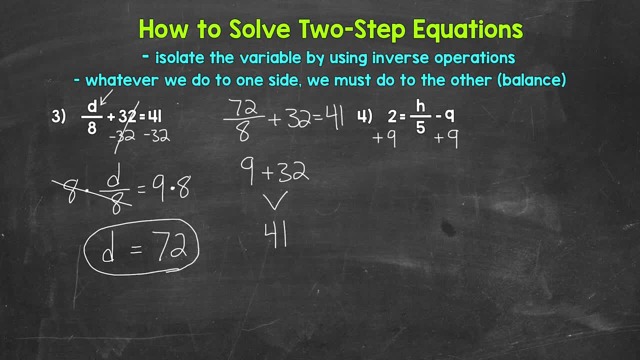 That means we need to add 9 to the left side as well, 9 to the left side as well. Now, on the right side of the equation, we are subtracting 9 and adding 9.. We are subtracting 9 and adding 9.. 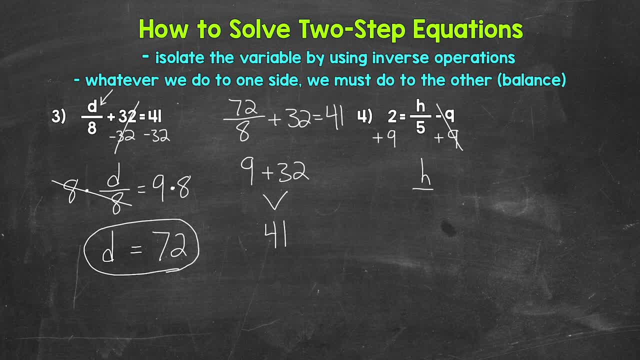 So those 9's cancel each other out. So we have h divided by 5 equals. So we have h divided by 5 equals. And then, on the left side, 2 plus 9 gives us 11.. 2 plus 9 gives us 11.. 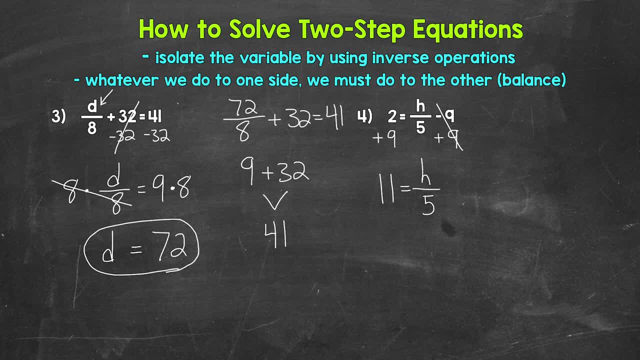 So h divided by 5 equals 11.. So h divided by 5, equals 11.. So we are dividing h by 5.. What's the inverse operation of division? What's the inverse operation of division? Well, multiplication. So we are dividing h by 5 equals 11.. 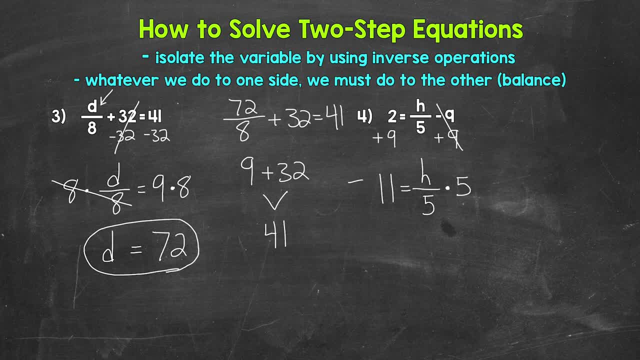 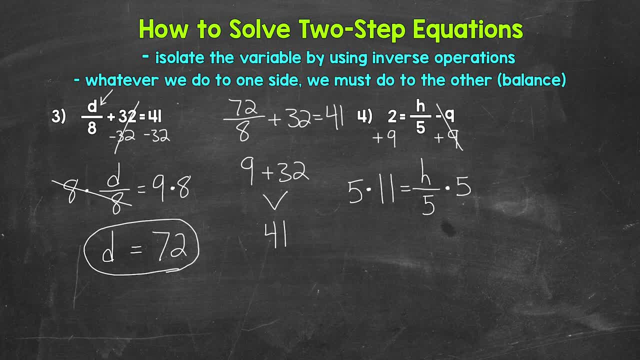 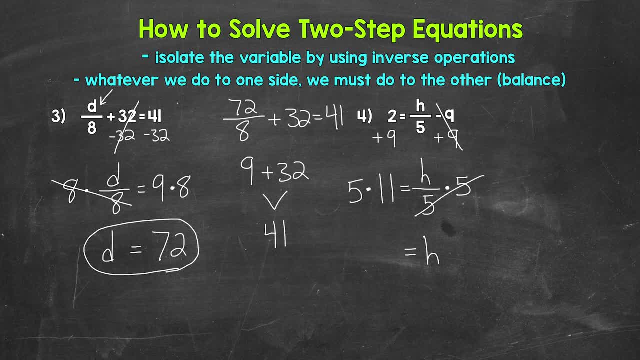 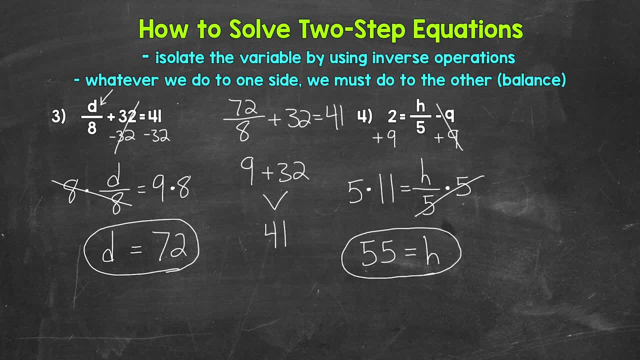